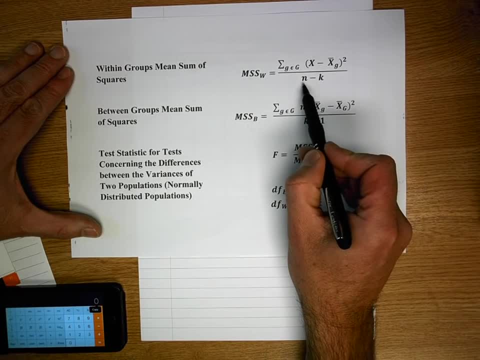 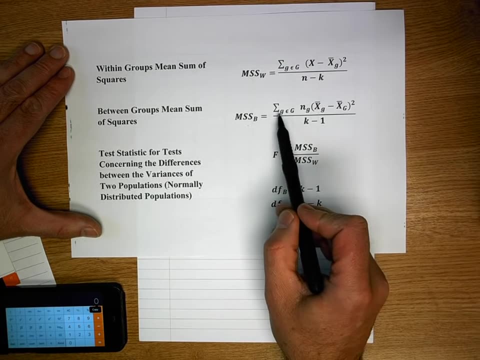 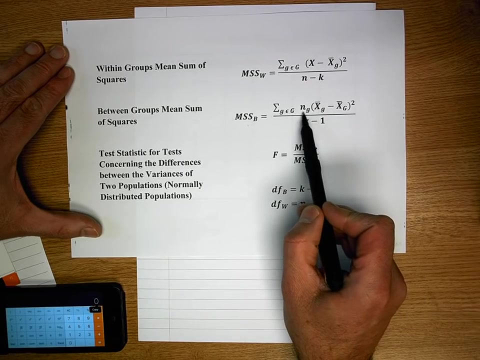 each group and square that We then divide by n minus k. n is the total number of variables and k is the total number of groups. The mean sum of squares between is again the sum for all values. so these are just individual values: g for all groups, capital, G. We're going to multiply the number in. 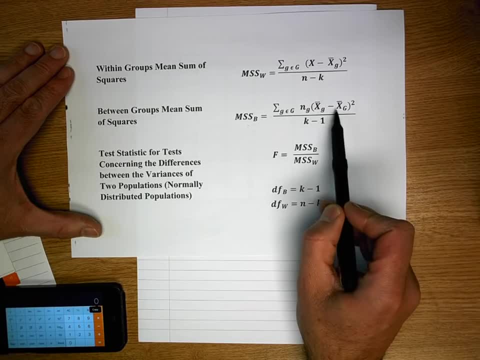 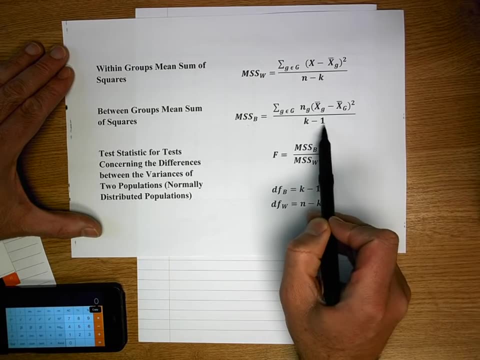 each group by the mean of each group, x bar small, g minus the mean of the overall grand mean, x bar capital, G squared, and we're going to divide that by k minus 1.. So, first off, there are some descriptive statistics that we need to determine before we can start. 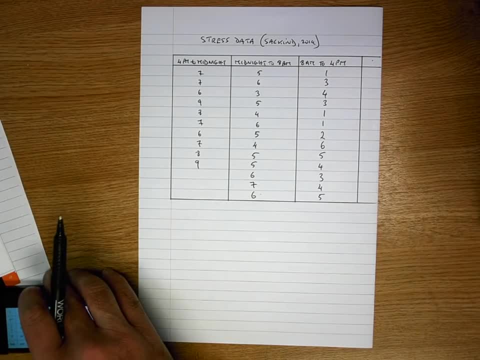 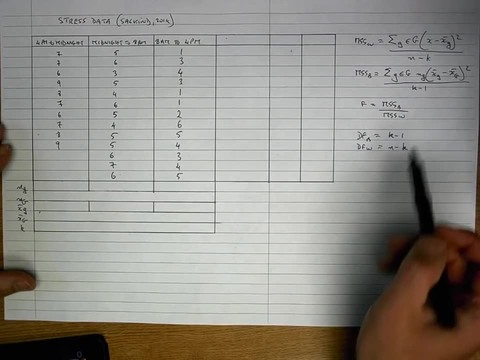 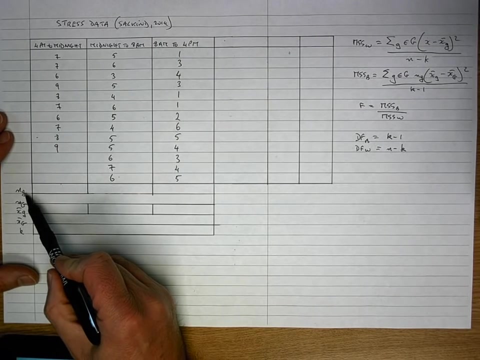 using plugging values into these formulae. So what I've done is I have first of all laid out my data as follows. I've got my formula just handwritten in over here on the right hand side and here are my three columns of data that we have just seen, And I need to calculate the number in each group. 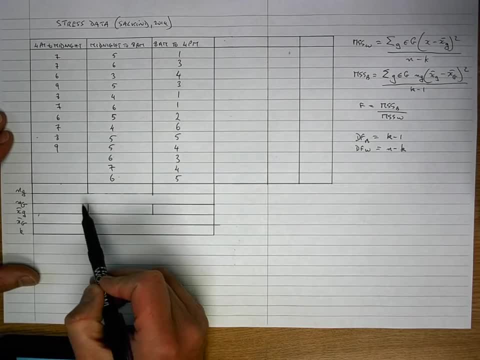 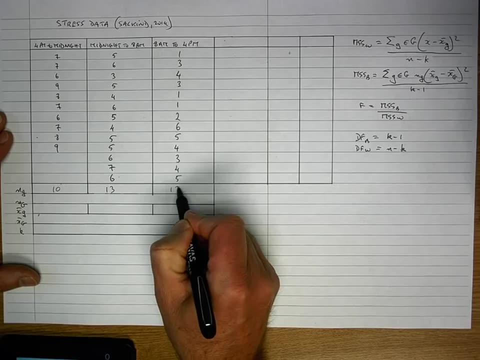 so n? g is the number in each group and n capital G is the overall number. So when I count up all these values here, I see I get 10.. Here I've got 13,. and for the third group I've also got 13. 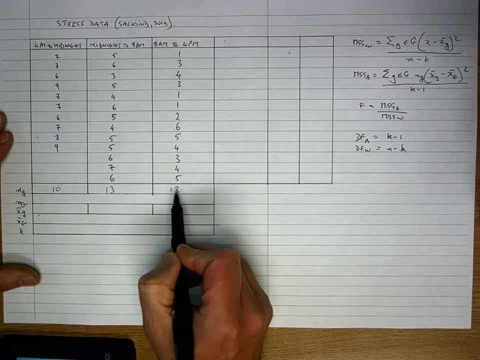 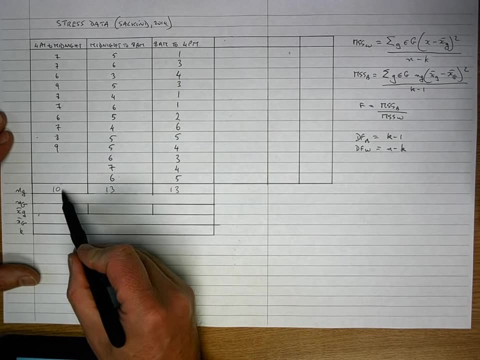 values. So n1 is going to be 10,, n2 is 13, and n3 is also 13.. n, capital, G is the number overall, the number of variables in all the groups combined. so that's going to be 10 plus 13 plus 13,, which is 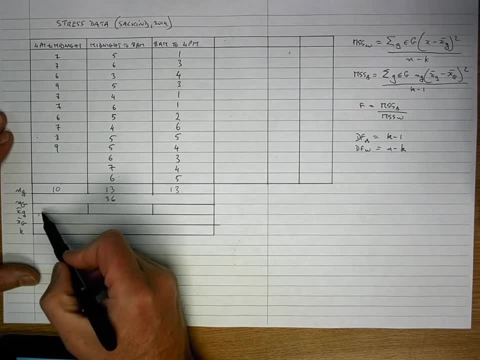 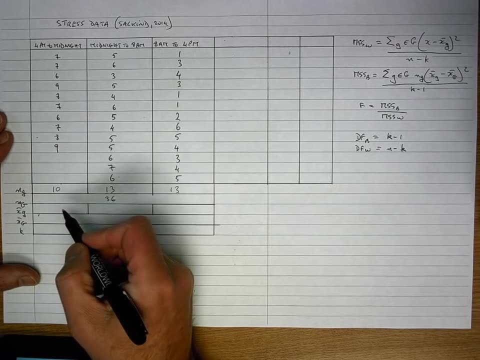 36.. And the mean. now we need to calculate the mean x bar for each of the groups. so small g, so that's going to be for the first group, all of these values added together and divided by 10,. 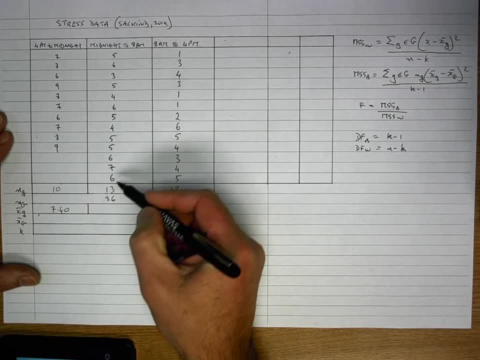 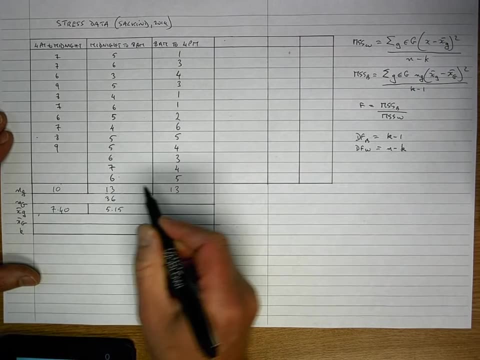 and when I do that, I get a result of 7.4.. When I calculate the average of the second group, add up all 13 values and divide by 13,. I get a result of 5.15, and when I do the same for the 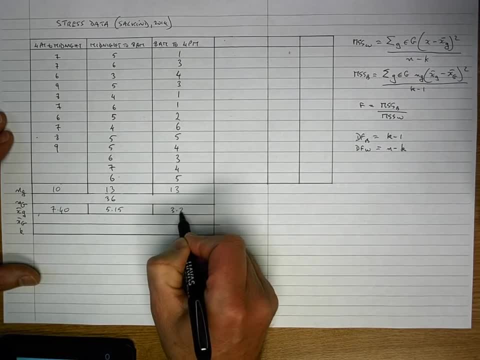 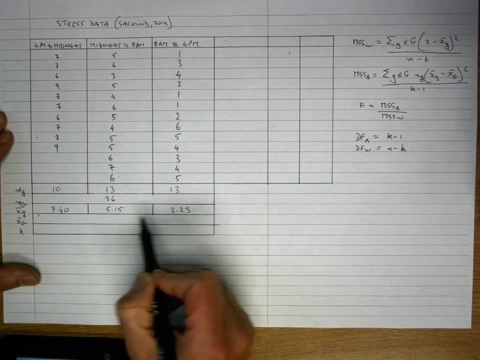 third group. add them all up, divide by 13,, I get a mean of that group of 3.23.. So x bar 1 is 7.4,, x bar 2 is 5.15, and x bar 3 is 3.23.. I also need to calculate the grand mean. so that's our capital. 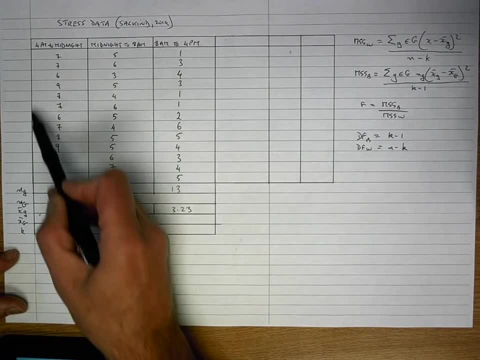 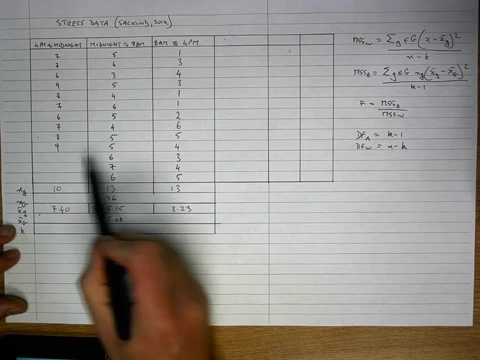 G, And so what we need to do, then, is take all 36 values here, add them all together and divide by 36, and when we do that, we get a result of 5.08.. If our sample sizes are the same- and they're not- 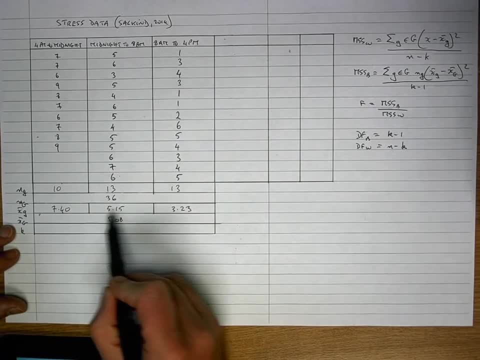 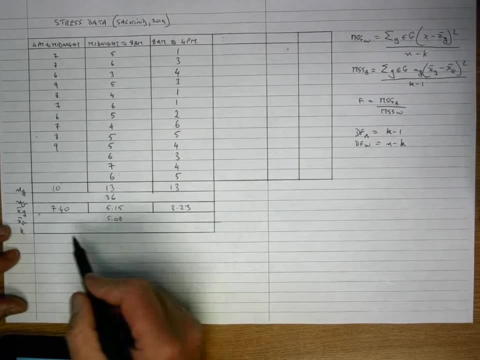 in my example here we could simply take the mean of the mean, so we can add those three values together and divide by 3 to get the mean of means. but that does not work if you've got different sample sizes. The final variable here is k, which is the number of groups. I've got three groups. 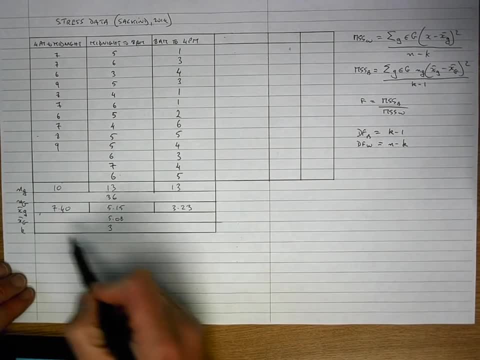 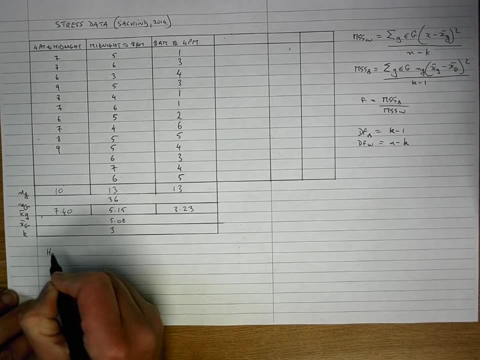 so I'm going to write down three in here. So this is typically what you would do when you're conducting an ANOVA test, so to set out your data like this. So let's start with our null hypothesis. So our H0 is that the mu of our first group- I'm going to call it group 1, is 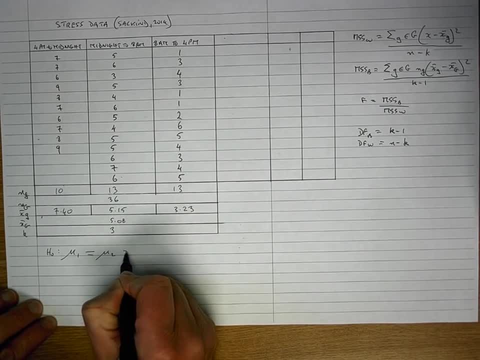 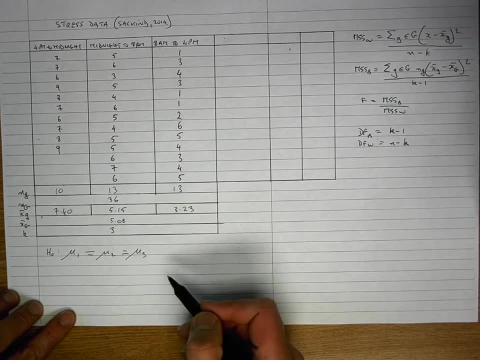 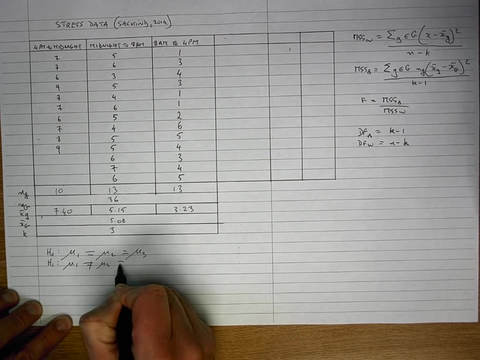 equal to the mu, the mean of the second group, which is equal to the mean of the third group. So my null hypothesis is that there's no difference between the populations in my example here. My alternate hypothesis- H1, is that mu 1 is not equal to mu 2, is not equal to mu 3.. So 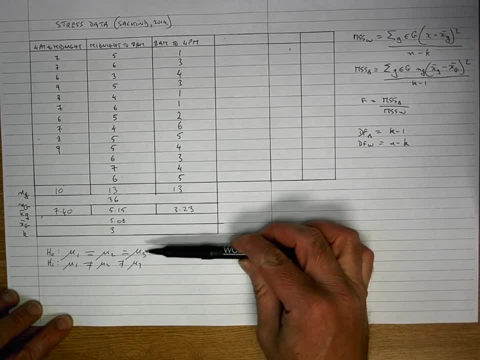 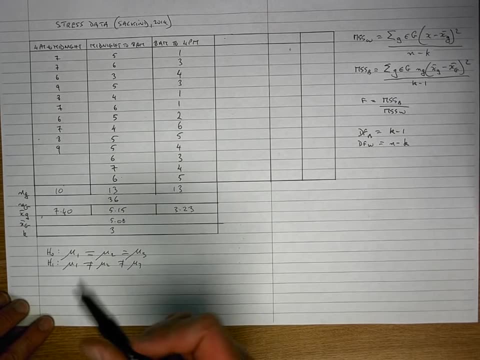 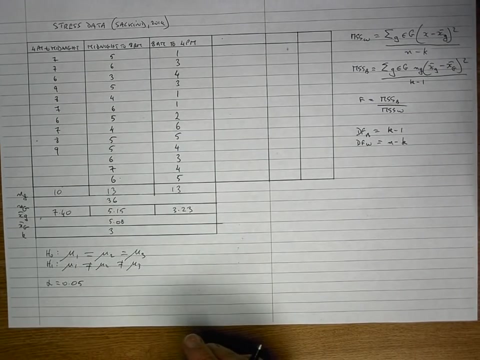 in other words, my null is that they're all the same, and my alternate hypothesis is that there's at least two of my groups have different levels of stress. I'm also going to work here with an ANOVA value of 0.05.. So we'll be coming back to that a little bit later on. So now the first. 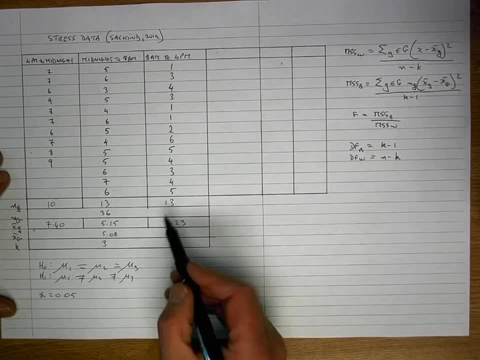 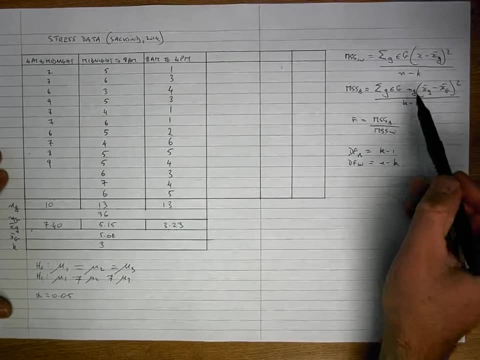 thing I need to do is to work out my formula So, based on these values over here on the mid-left hand side, I can plug a lot of these values into my formula that I need over here on the right side. But one of the things you can see I need is I need to determine x minus x bar squared for each value. 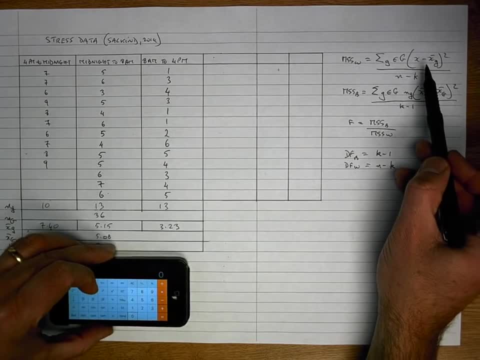 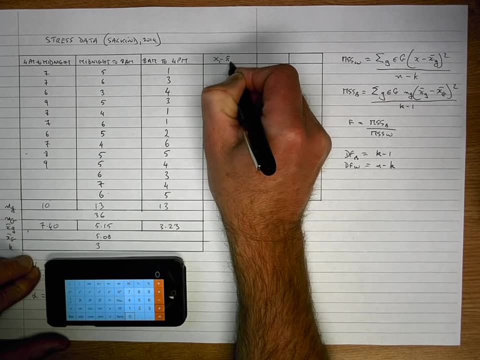 in each of the groups. So let's go ahead and go about doing that. I've got three columns set up here, So I'm going to have x bar 1 minus x1 minus x bar 1 squared, So that's going to be the first. 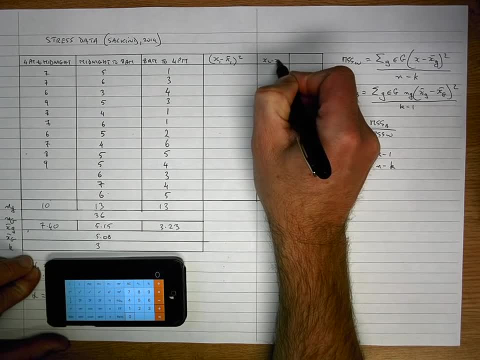 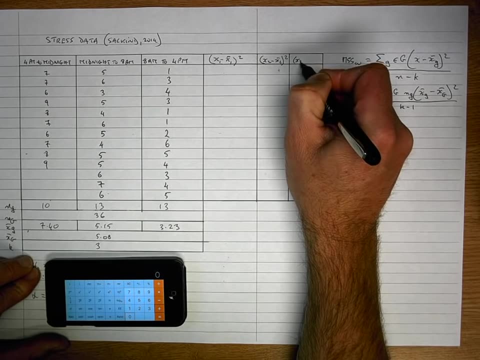 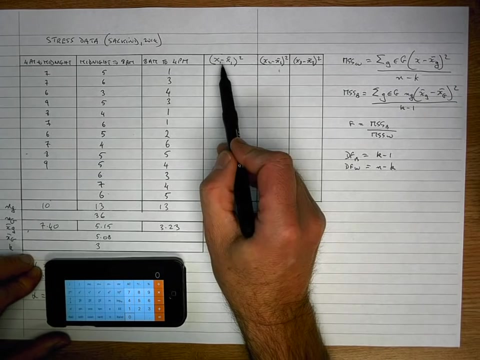 group of 10 values here: x2 minus x bar 2 squared. And that's going to be the calculations for the second group, and the third group will be designated x3.. Minus x- bar 3 squared. So now I need to populate all these values here, So to calculate x1 minus x. 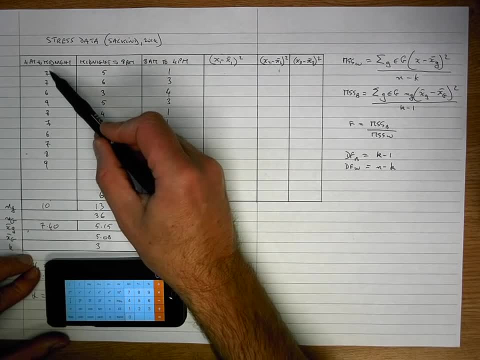 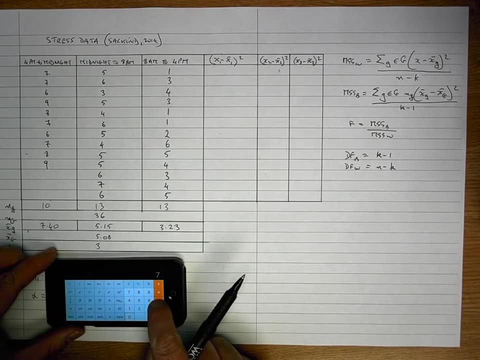 bar 1 squared for the first value of 7 here. so that's going to be 7 minus the mean, which is 7.4, and we square the result. So let's go ahead and do that. So we've got 7 minus 7.4.. That's equal to. 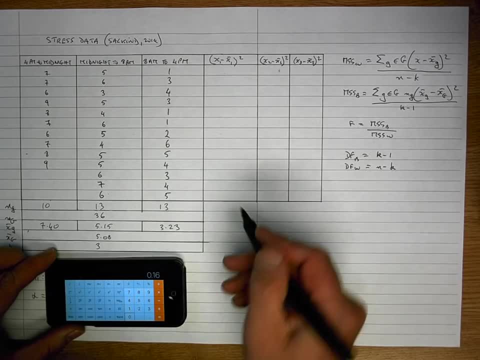 minus 0.4.. And we square that and we get a result of 0.16.. I can see in my data that my second group is going to be the first group of 10 values. So I'm going to have x bar 1 minus x bar. 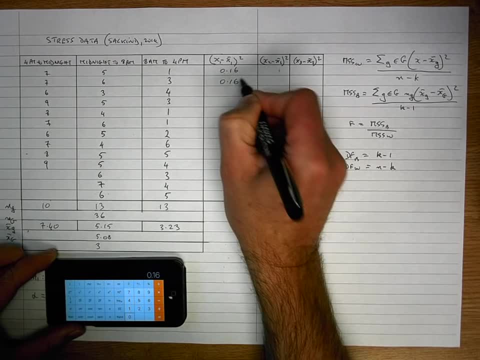 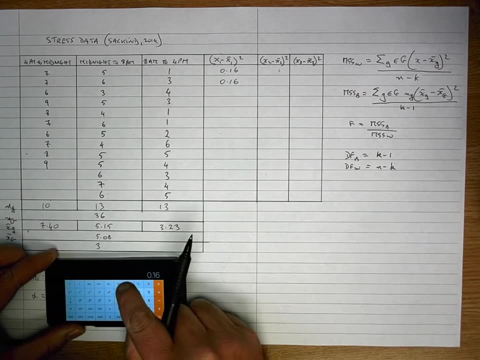 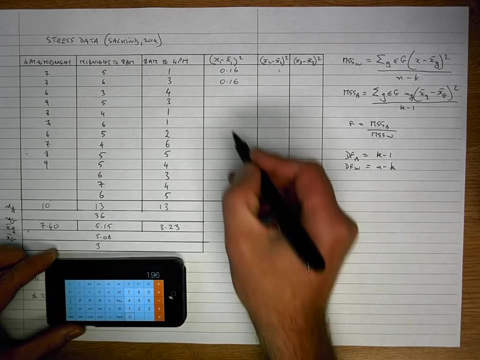 1 squared here. So 6 is the next value. So 6 minus the mean 7.4, is equal to minus 1.4.. We square that value and the next one is 1.96, and so on, And we do that until we get down to the last value. 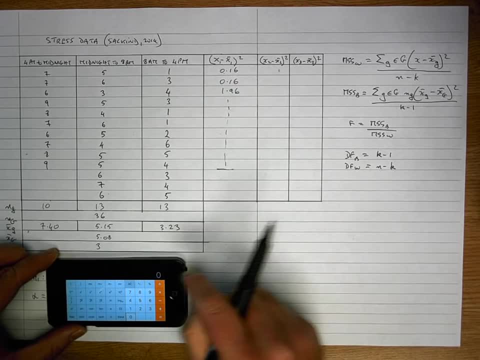 here for the 10th value in this column. We now move over to the next column. We're going to do the same thing for the second group of 10 values. So we're going to have x1 minus x bar 1 squared. 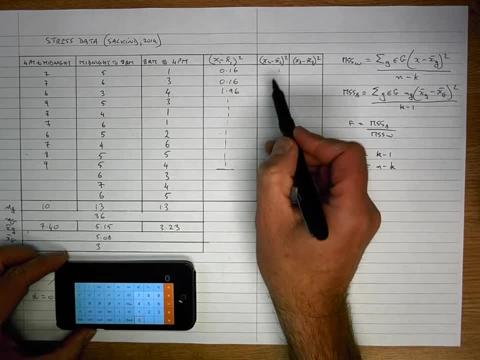 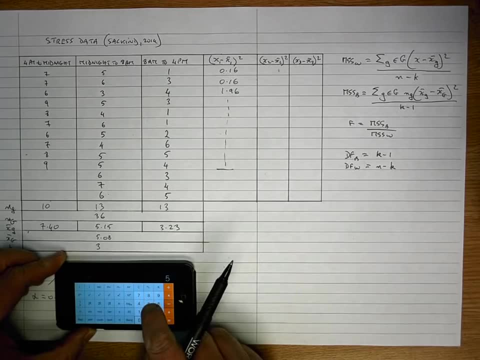 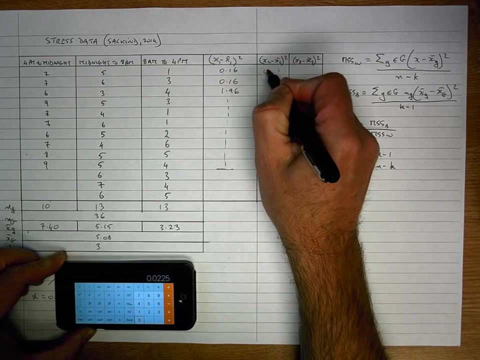 So that's our group 2.. So our first calculation here is 5 minus the mean of 5.15, and we square that value. So 5 minus 5.15 equals 0.15 minus, and we square that and we get 0.02 rounded. 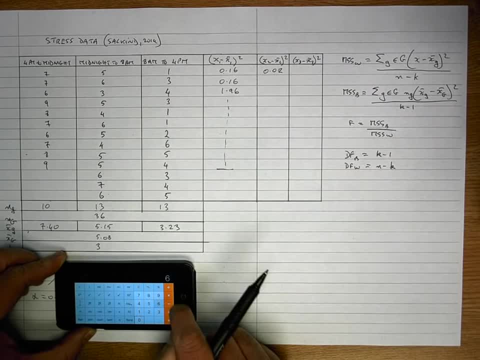 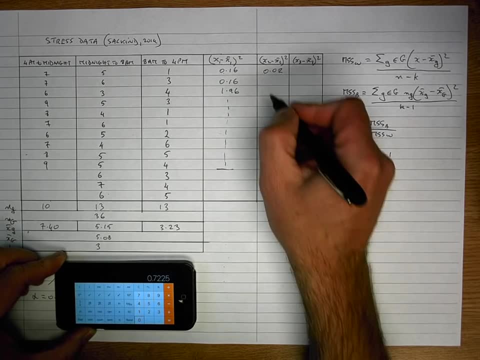 My next value is 6 minus the mean. So 6 minus 5.15 equals 0.85. squared is 0.72.. 0.72.. And of course we keep doing that until, in this case, going down right down to the end. 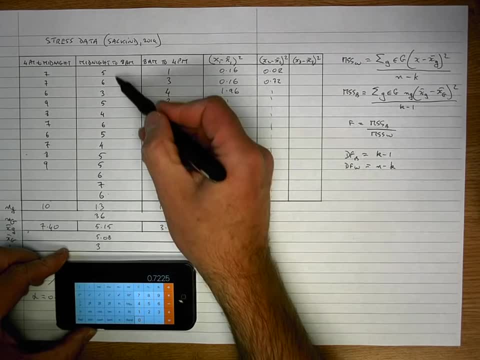 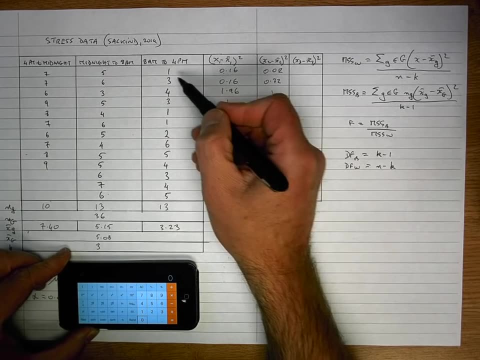 all 13 values. to work out x2 minus x bar for each of these values here And just to confirm, we do the same in the third value here. So this is x3 minus x bar 3.. So our first x3 is 1. It's. 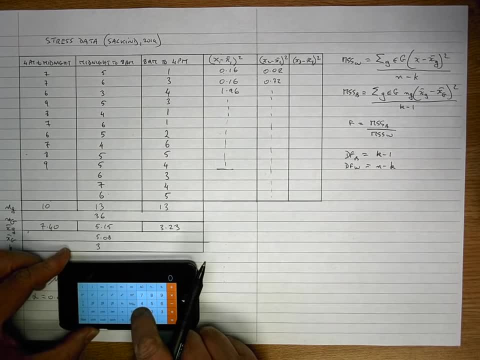 going to be minus 3.23 squared, So let's do that. 1 minus 3.23 is equal to minus 2.23.. We square that. Whoops, I need to do that again. 1 minus 3.23 is equal to minus 2.23 squared. So that's. 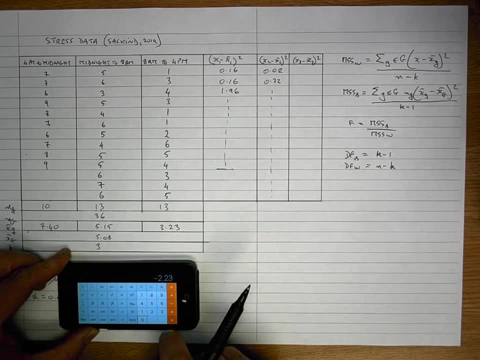 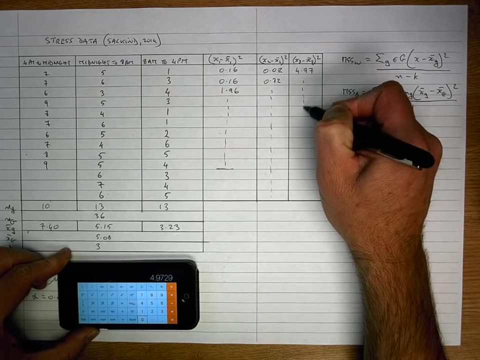 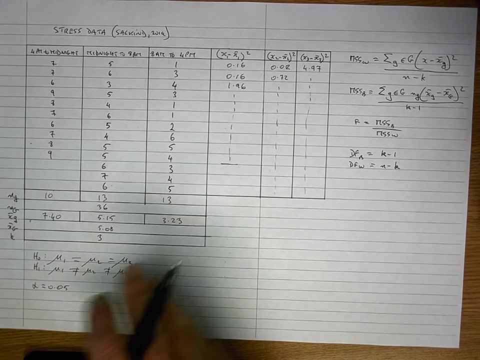 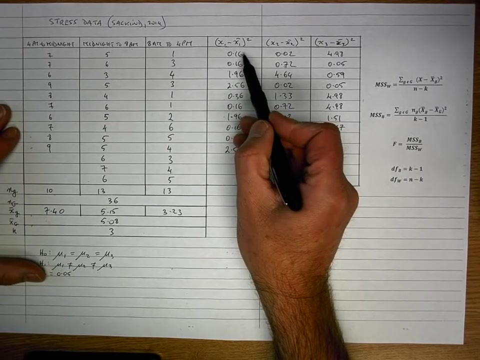 minus 3.23 is equal to minus 2.23 squared. It gives me 4.97 rounded. And I keep doing that then for each of the values here in this column. So earlier I have actually filled out all those values And here they are in my sheet, So I've got all of the x minus x bar squared for all my. 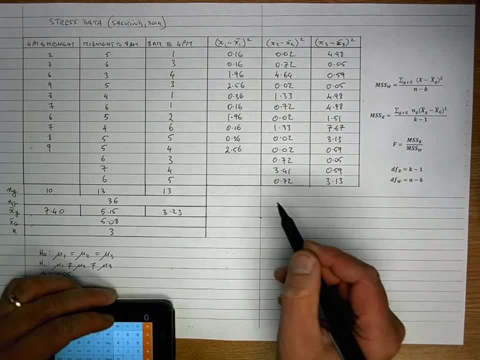 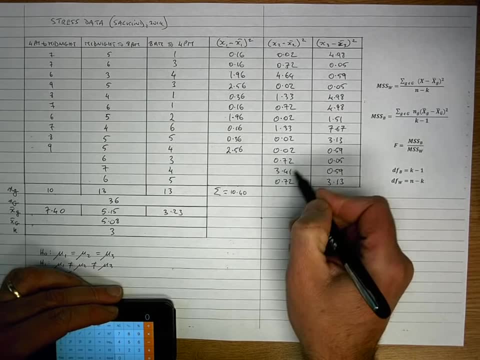 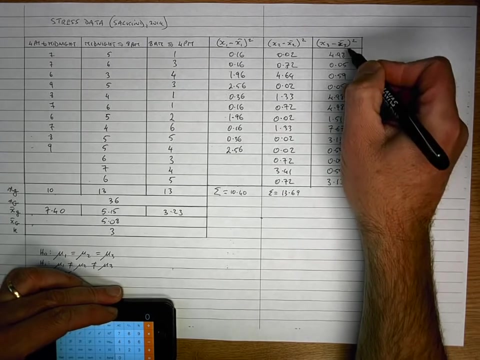 first group, second group and third group. And now I need to sum them all up. So the sum, just by adding up all of those values there, that's equal to, you get 10.4.. Add up all the second ones here, This is sum is equal to 13.69.. And simple addition of all these third group here. 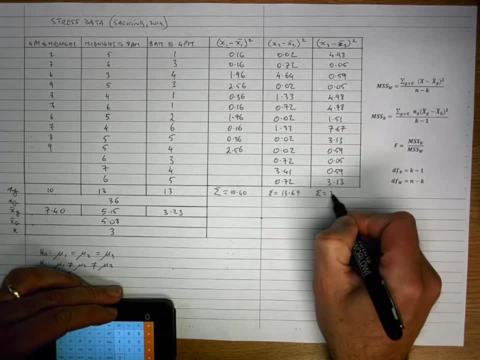 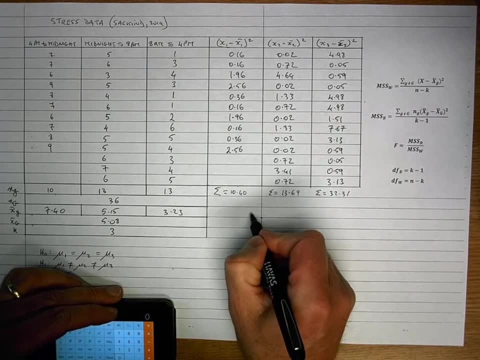 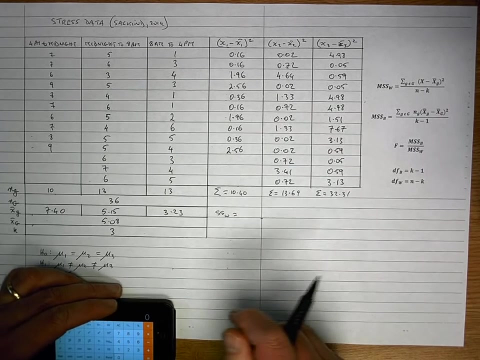 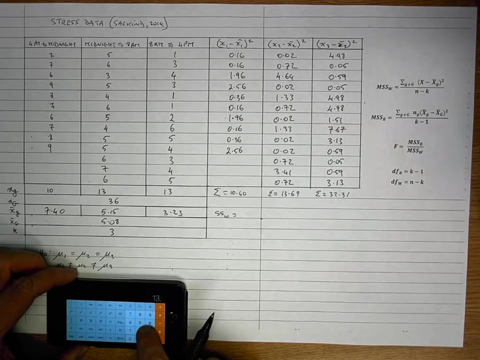 is that our sum is going to be equal to 32.31.. So these are our individual group sums of squares. So when I add these two tree groups together, so I will get my sum of squares And I'm working on the sum of the three of these figures added. So let's go ahead and do that. So 10.4 plus 13.69 plus. 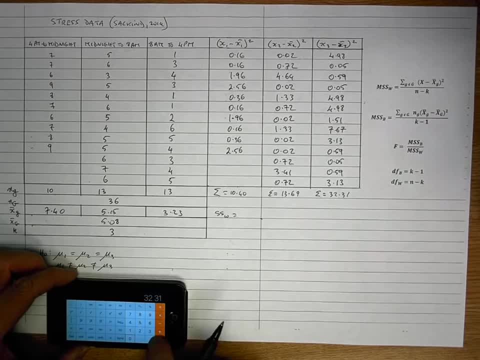 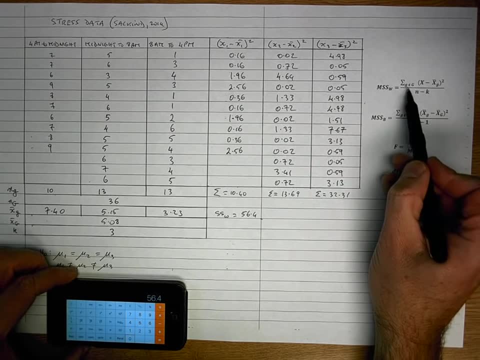 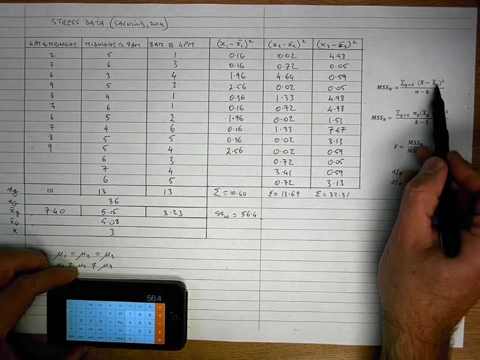 32.31 is equal to 56.4.. So that is effectively that is the top part of our formula over here. So we've now worked out the sum of all of the individual values for all of the groups, x minus x bar squared for each one. Add them all together And now we need to divide. 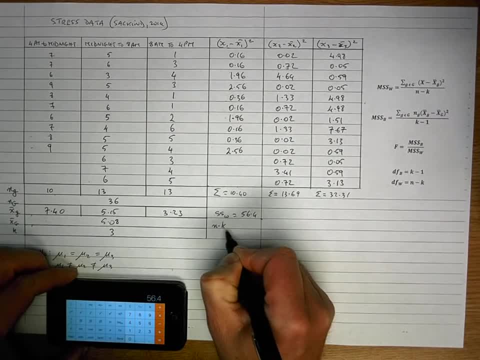 by n minus k. So n minus k, okay, that's equal to n, which is 36, the grand n minus k, which is three. So 36 minus three will give us 33.. So our mean sum of squares, then mean sum of squares. 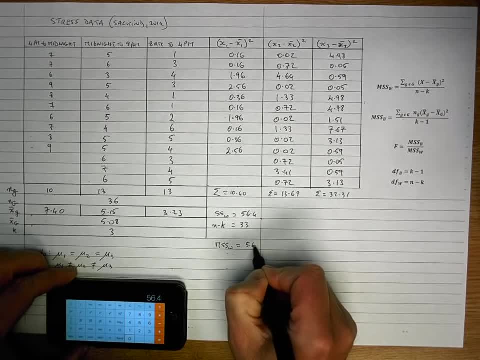 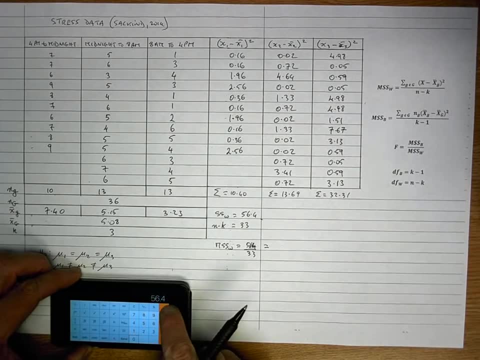 within is equal to 56.4 divided by 33, which is equal to. let's do that 56.4 in my calculator divided by 33 is equal to 1.71.. Rounded So, my mean sum of squares w within is 1.71.. I have now calculated the denominator in my 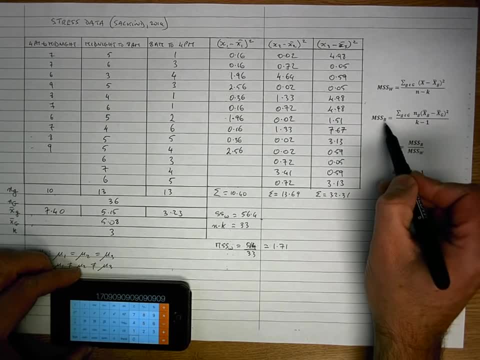 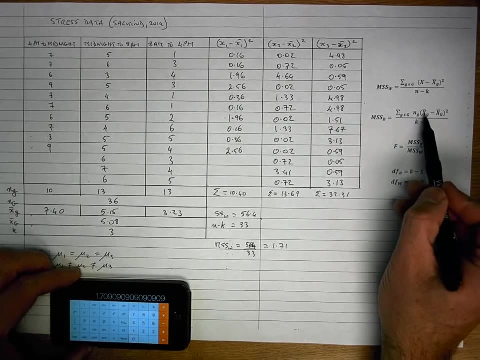 f formula over here. Now we need to go over and calculate the mean sum of squares between- And we can see in our formula here that we need to for each of the groups. so we've got three groups, so we're going to take the mean of each group and subtract the grand mean square it. 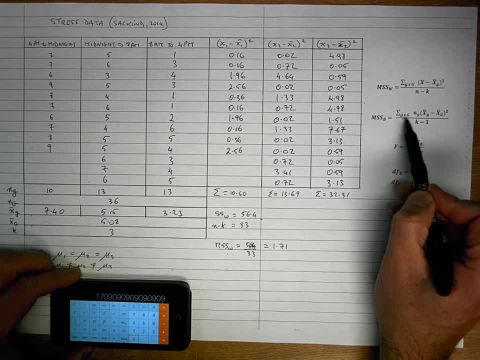 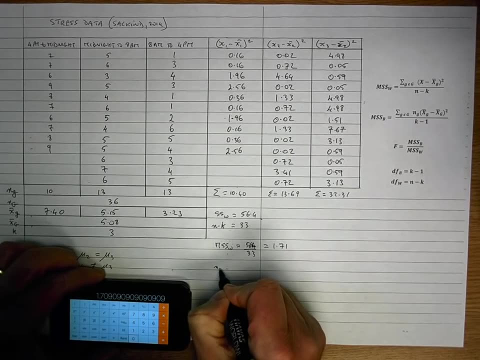 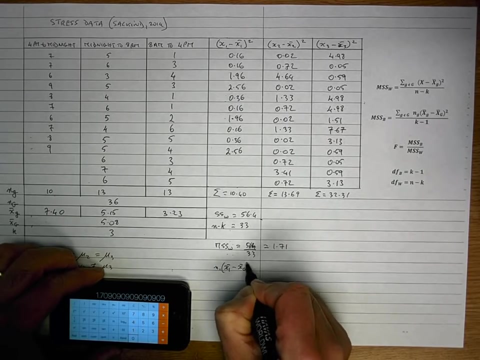 and multiply it by the number of each group. We're going to do that for all groups. Then divide by k minus minus one. So work out our formulas here for this. So n one for the formula is equal to first group. this is equal to x bar one minus x bar, grand g squared And we're going to get a value. 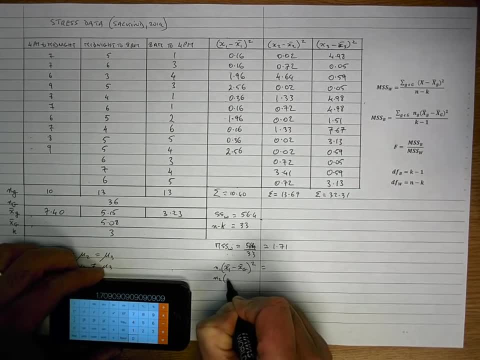 for that. Our second group is going to be n2 times x bar two minus the grand mean, again squared. And the final group- we have three groups here- x bar three minus x bar, grand squared is equal to: and if I had four or five groups I would keep doing this. So now all the values I need for. 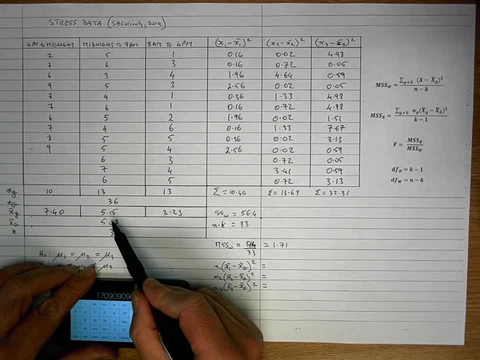 these individual calculations are going to be- I'm going to keep doing this, So I'm going to keep- are taken from my table that I created earlier on. So let's fill these out: N1 is 10,. n2 is 13,. 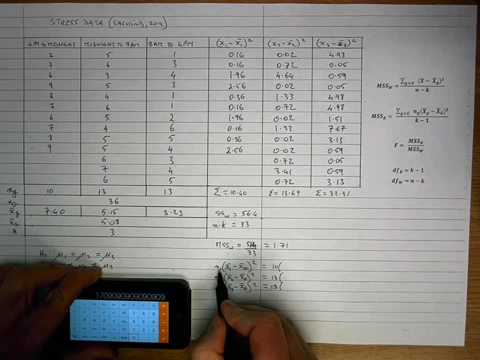 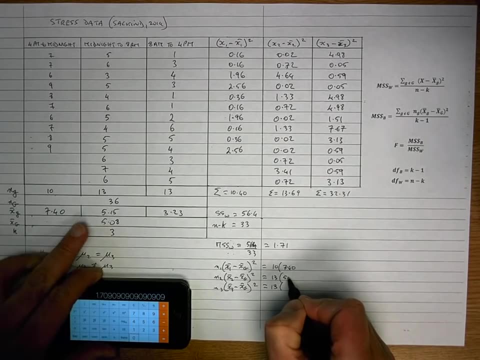 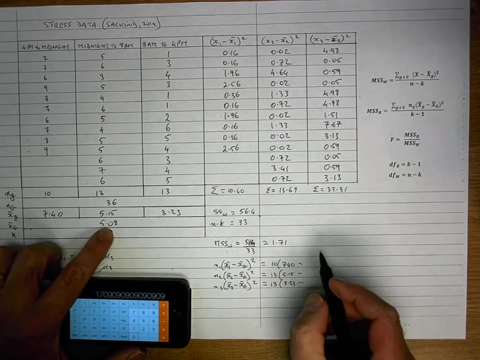 and n3 is also 13.. So that's the first part of each formula: n1,, n2,, n3.. x bar one is 7.40,, x bar two is 5.15, and x bar three is 3.23, minus the grand mean, which is 5.08 in each case. so 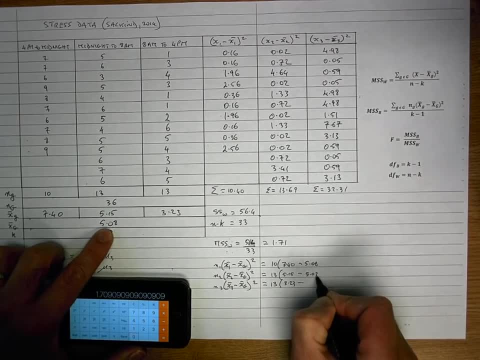 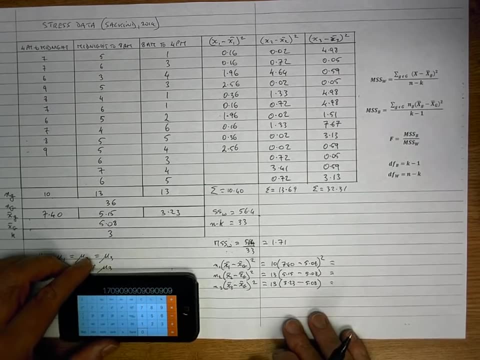 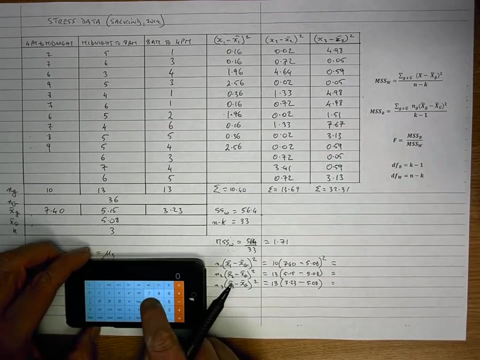 5.08,, 5.08,, 5.08.. 08, and we square that. so let's work out what each one of these is. so I'm going to do the middle bit, first square and then multiply by n. so 7.4 minus 5.08 is 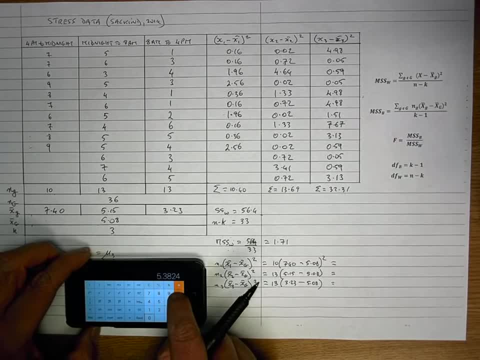 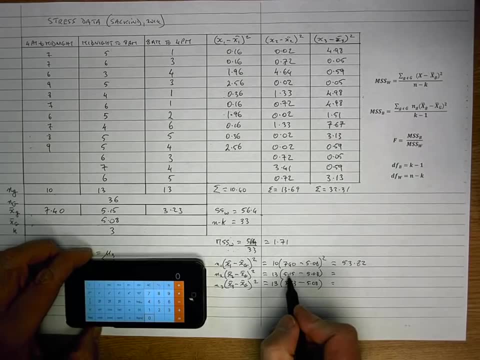 equal to 2.32. square that, and then multiply by 10, that's equal to 53.82. the next one is 5.15 minus 5.08 squared. then multiply by 13 minus 5.08. equal square that and multiply by 13 is 0.06. the last 1: 3.23 minus 5.08. 3.23 minus 5.08. 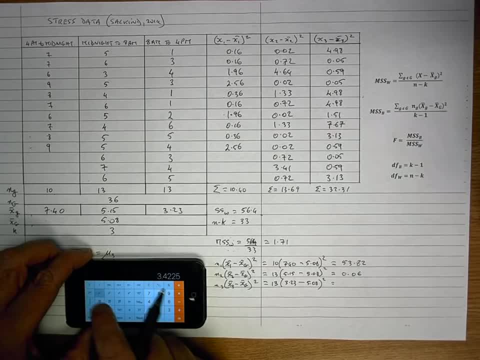 equals minus 1.85. we square that and multiply by 13.. Multiply by 13,, and that gives us 44.49.. So now we need to sum all of these together. So the sum of these three here is equal to just let's add all of those up. 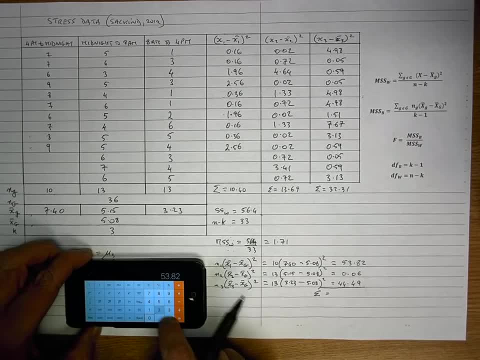 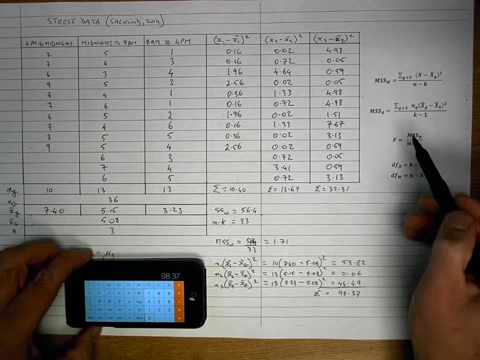 So 53.82 plus 0.06 plus 44.49.. That gives us a total, the sum of all of these values here, of 98.37.. So what I have done in my formula here is that I have worked out the top line for the mean sum of squares. 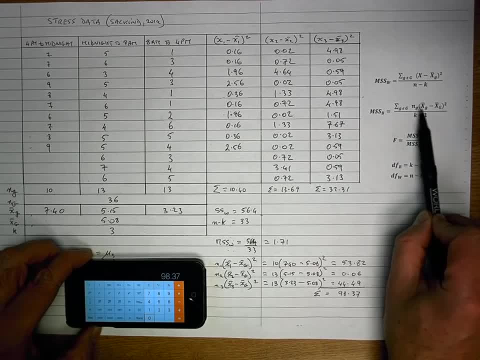 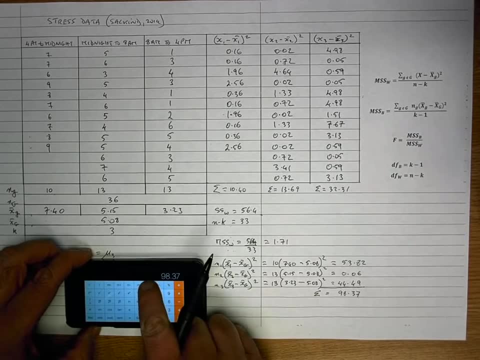 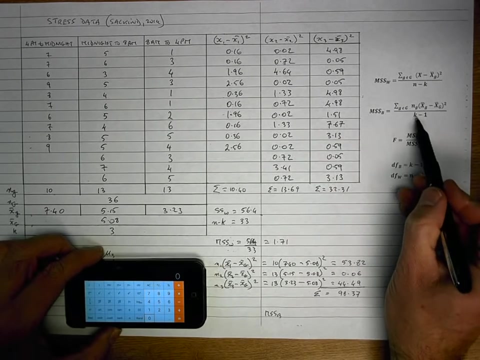 between all of the values. add them all up for each group, the mean of each group minus the grand mean squared. So that's the total here of 98.37.. So now I need so my mean sum of squares. then my formula is: I take that value and divide by k minus 1.. 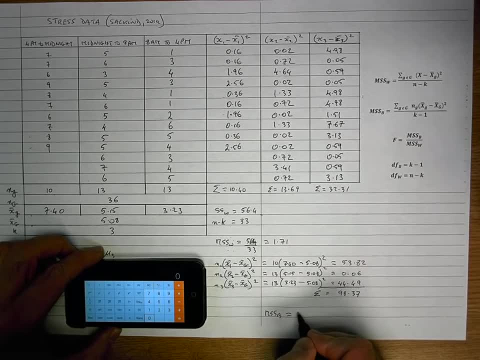 Now k is 3, so we need to divide that 98.37 divided by k minus 1,, which is 3 minus 1., Which is 2, and that equals 2, so 98.37 divided by 2 is equal to 49.19 rounded. 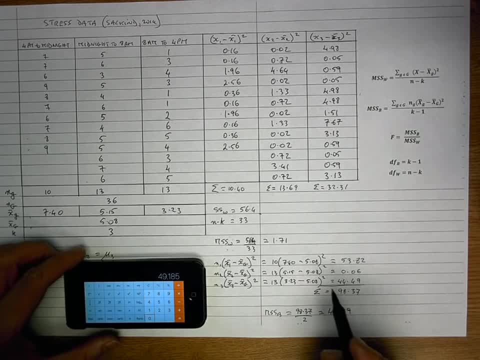 So 49.19 rounded represents my mean sum of squares between. So I have my mean sum of squares within up here. I have my mean sum of squares between down here and my F statistic then is my mean sum of squares between divided by my mean sum of squares within. 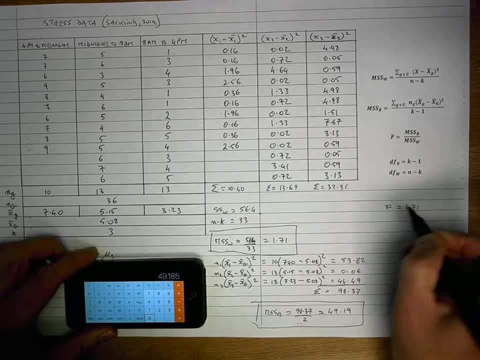 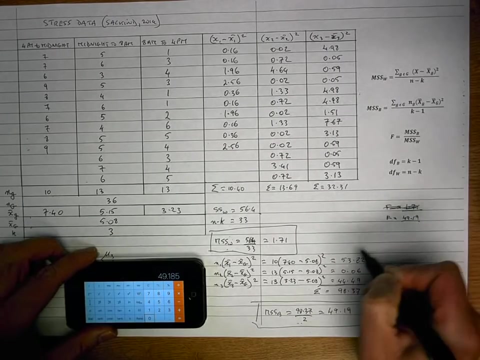 So that's going to be 1.7.. 1,, which I've got from here, divided by 49.19.. Sorry, it's the other way around, isn't it? Yep? mean sum of squares between is equal to 49.19 divided by 1.71.. 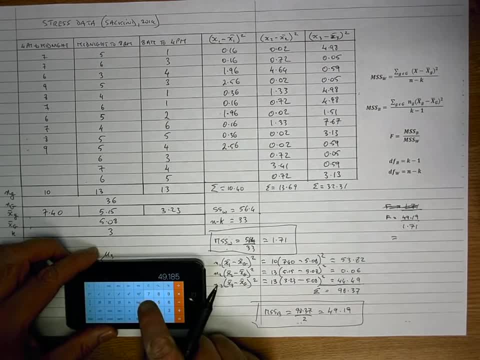 So let's see what that is. So 49.19 divided by 1.71 is equal to 28.77 rounded: 28.77. 28.77. 28.77. 28.77 rounded. So that's my F statistic. 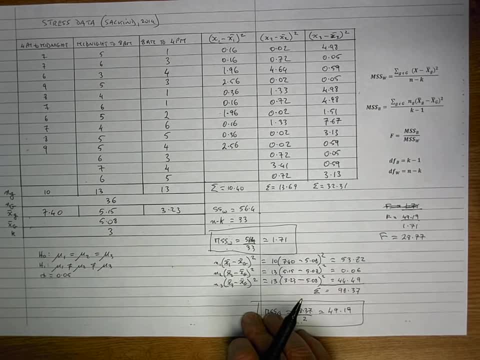 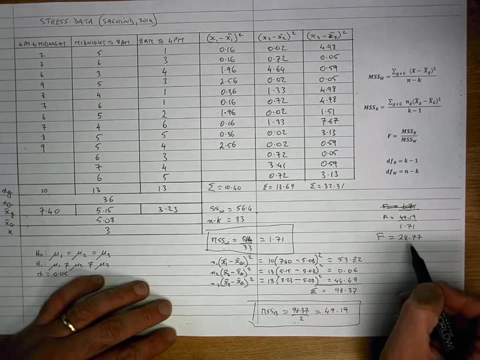 So that's calculations done for now. I've got a couple of small ones left to do. My F statistic is 28.27.. I now need to look up some tables to determine if this represents a significant difference between the three groups or not. 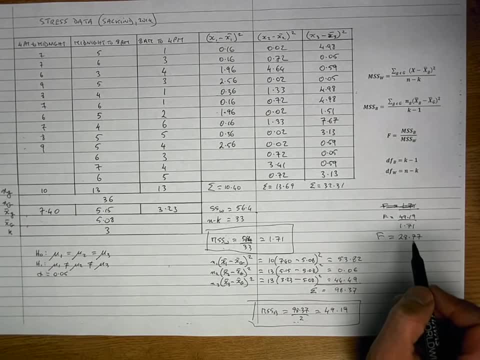 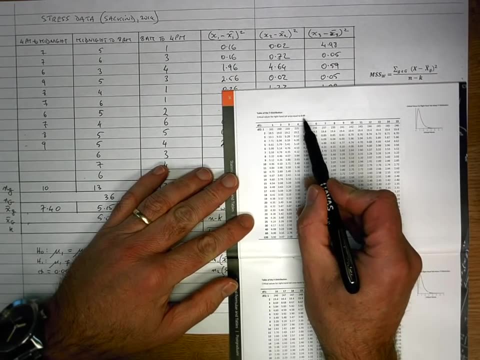 To do this, I need to check my F distribution. The F distribution I'm looking at is the 1, 4.. And the 2, 4, alpha value of equal to 0.05.. And so I need to know what column and what row to choose here. 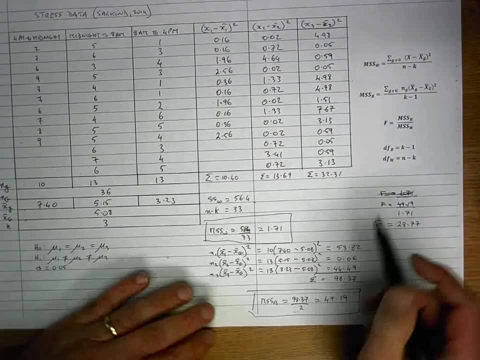 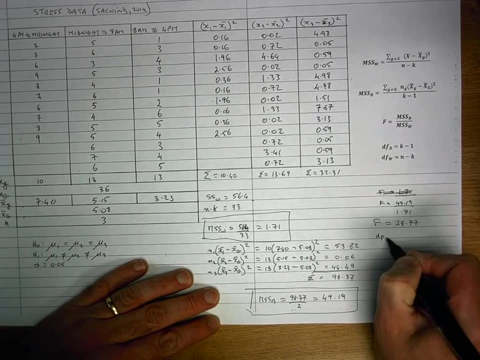 So I'm going to go back now to my formula over here. My degrees of freedom between is equal to K minus 1.. So that's 3 minus 1.. So my degrees of freedom between is equal to 3 minus 1, which is equal to 2.. 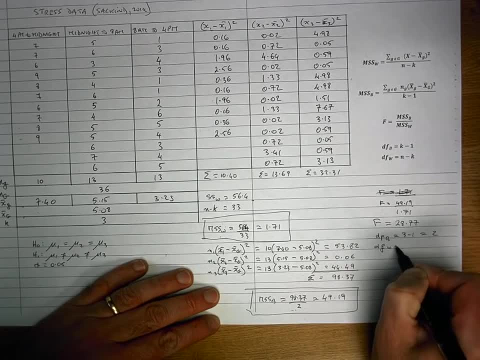 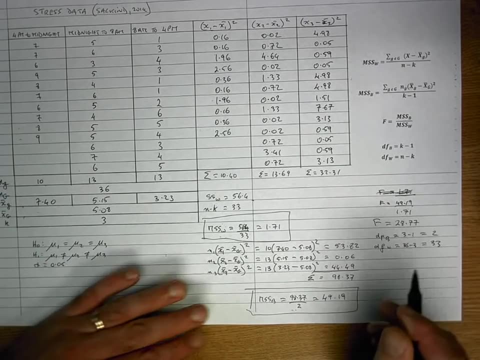 And my degrees of freedom within is equal to N, which is 36, minus K, which is 3.. So 36 minus 3,, which is equal to 33.. So the degrees of freedom within and within are the same. It's the same. 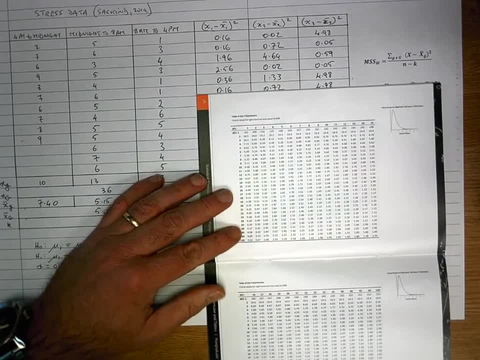 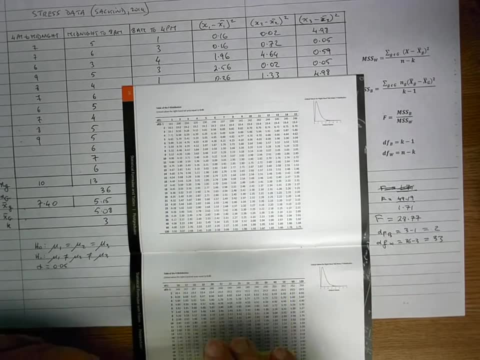 It's the same. The degrees of freedom between represents the column. so that's going to be a value of 2, so I'm going to go down this column here- a value of 2, and with my ruler here I'm going to mark out the line nearest to 30,. 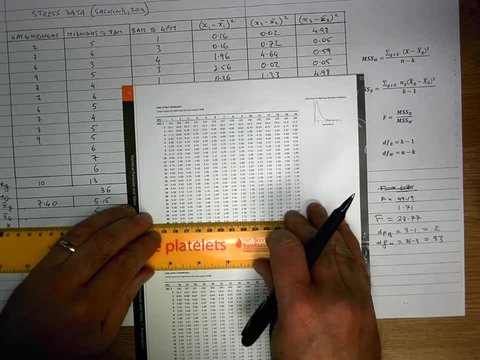 so in my version of the tables I don't have a figure for 33, so I'm going to go to the nearest figure, which is 30, and that gives me a critical value, my F critical value of 3.32.. 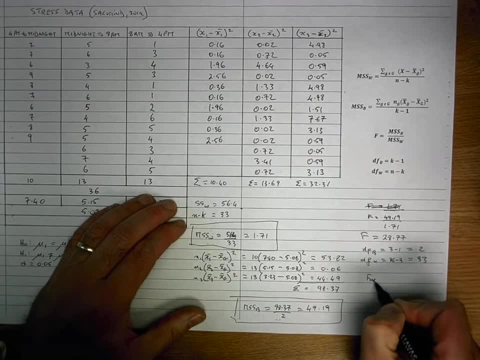 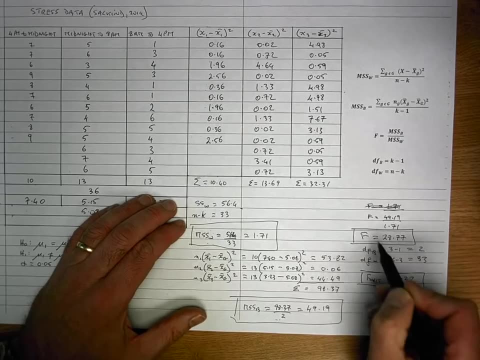 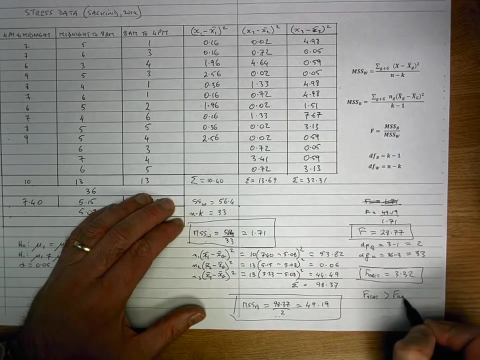 So my F critical is equal to 3.32.. I can see from my F value up here and my critical value here that my F stat, my F statistic, is greater than my F crit, my critical statistic. therefore, I have enough evidence to reject the null hypothesis. 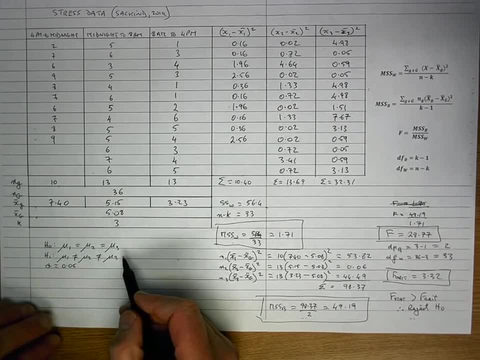 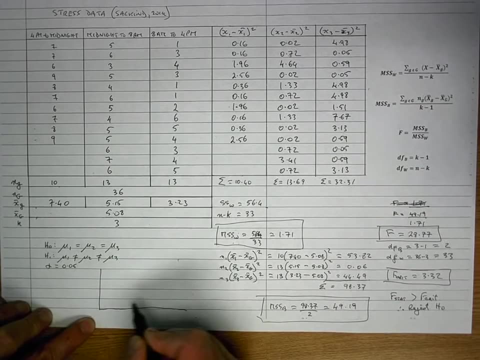 So coming back over here to the left-hand side, to my null hypothesis, my F stat is greater than the F crit. therefore I reject, so I draw my F distribution here. it's going to be something like this, with the tail over here down at the end: